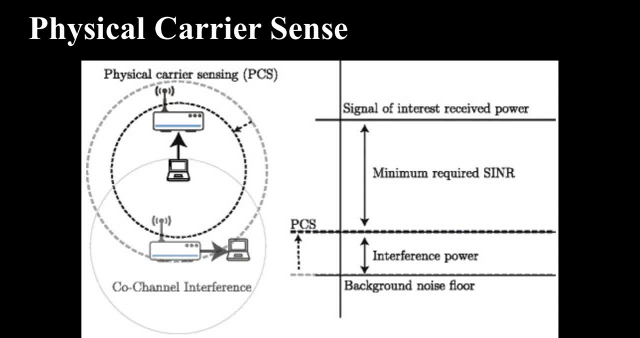 detect. SD ED functionality is based upon raw RF energy. When an energy level detected in the channel crosses a certain threshold for a certain period of time, the busy medium indication will be triggered. On the other hand, SD is nothing but preamble detection. 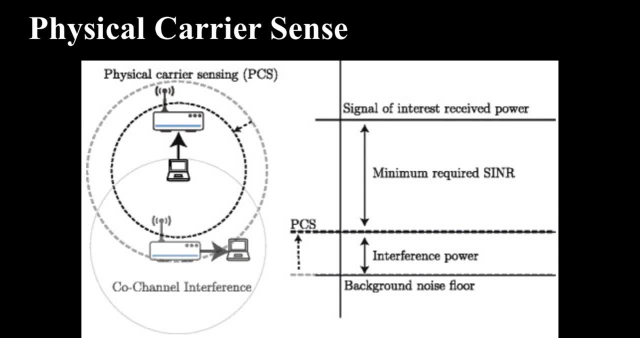 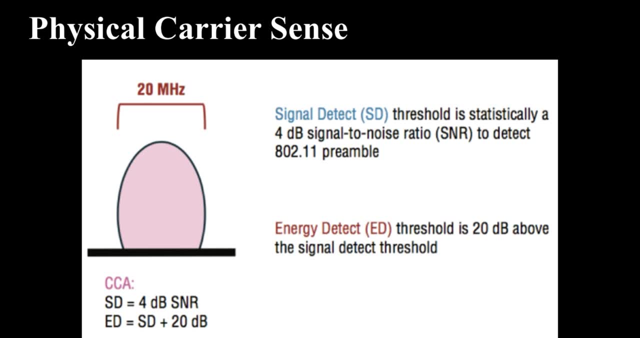 used to trigger the CCA mechanism to indicate a busy medium. CCA indicates a busy medium when the start of a valid OFDM transmission is received at a level equal to or greater than the minimum modulation and coding rate sensitivity, which is minus 82 dBm. this is 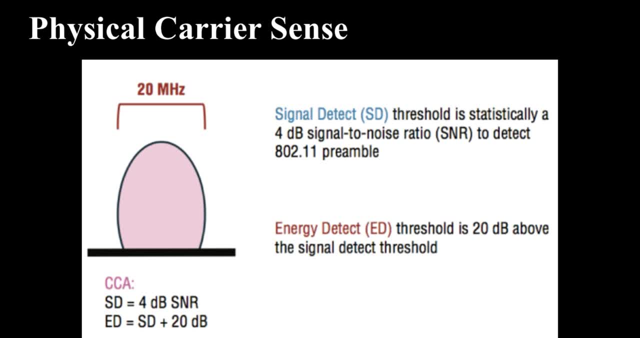 an example of signal detect. If the preamble of the frame is missed, the CCA holds a busy medium for any signal: 20 dB above the minimum modulation and coding rate sensitivity, which equates to minus 62 dBm. this is an example of energy detect. CCA sensitivity is much. 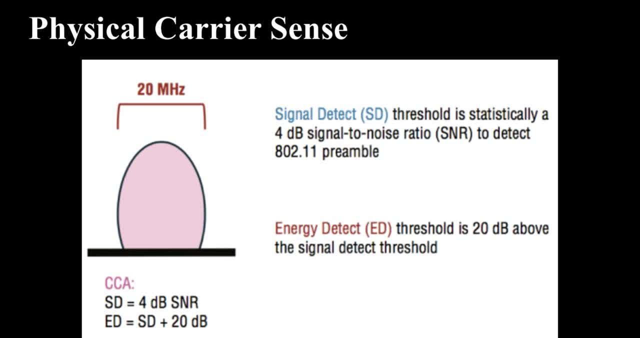 higher when the frame header is received and processed correctly. The sensitivity threshold for RF noise, including frames whose header was not processed, is much lower, at minus 62 dBm. Thus it takes a much stronger signal to indicate a busy medium when energy detect. 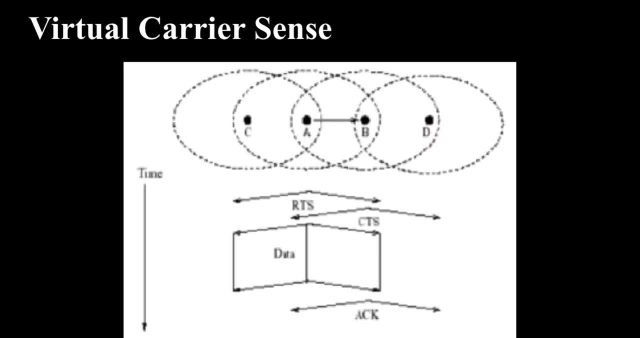 is used instead of signal detect. VCS is performed by means of the network allocation vector, NAV, which is a timer that is set using the duration values in the MAC header of a frame. Each frame contains a duration value indicating the time required for a station. All stations use these duration values. 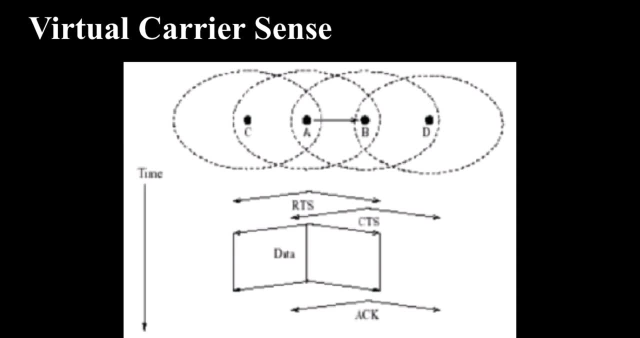 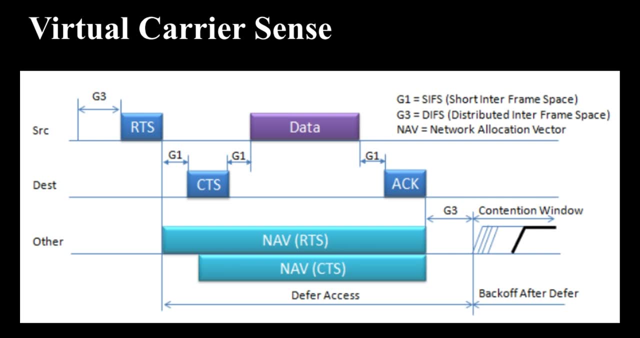 to set their NAV and then they count down the NAV timer waiting for the medium to become available. When stations read the duration value in a frame, they count down the NAV timer waiting for the medium to become available. When stations read the duration value in a frame, they count down the NAV timer waiting for the. 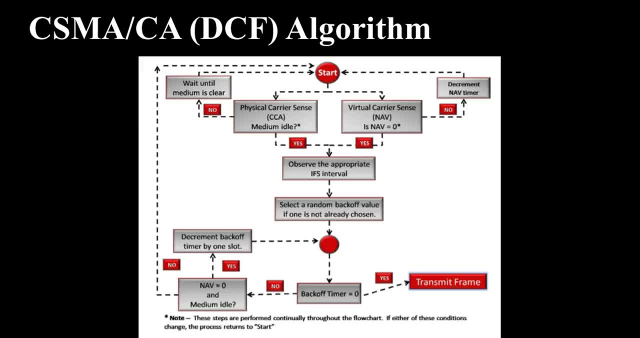 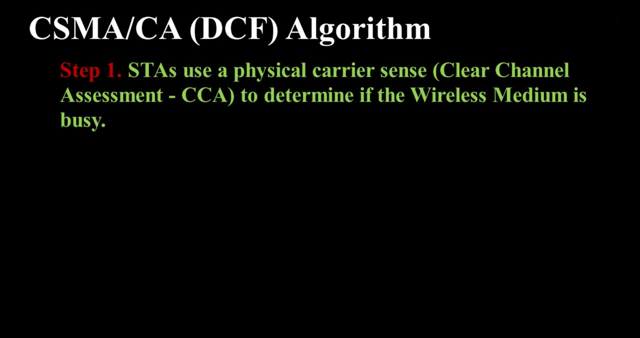 medium to become available. When stations read the duration value in a frame, they set their NAV timer accordingly and count down this duration. CSMACA DCF Algorithm. Let us discuss the DCF algorithm steps in detail. Step 1. Stations use a physical carrier sense to determine if the wireless medium 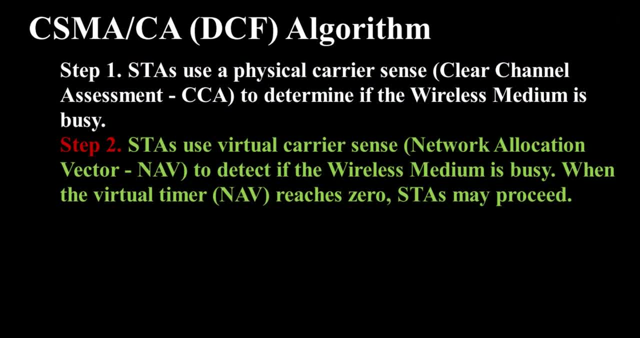 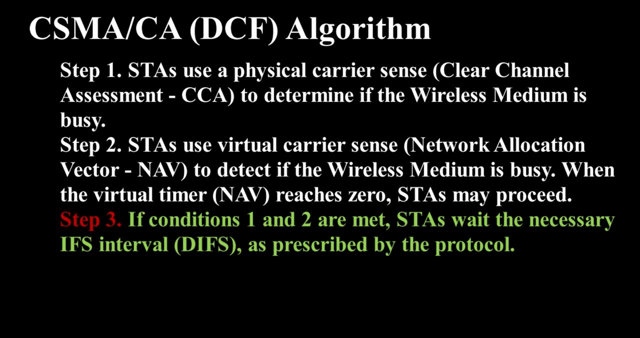 is busy: Step 2. Stations use virtual carrier sense to detect if the wireless medium is busy. When their NAV reaches zero, stations may proceed. Step 3.. If conditions 1 and 2 are met, stations wait the necessary inter-frame space interval. 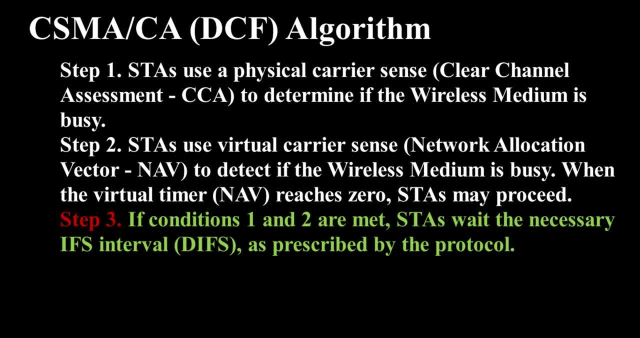 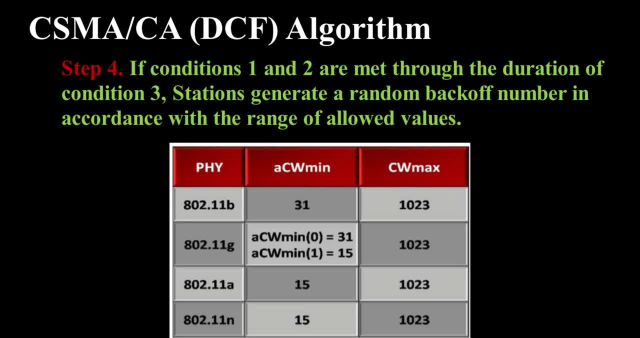 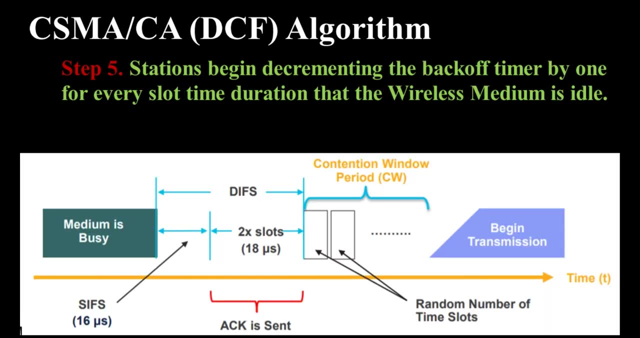 as prescribed by the protocol. Step 4. If conditions 1 and 2 are met, through the duration of condition 3, stations generate a random backoff number in accordance with the range of allowed values. Step 5. Stations begin decrementing the backoff number. 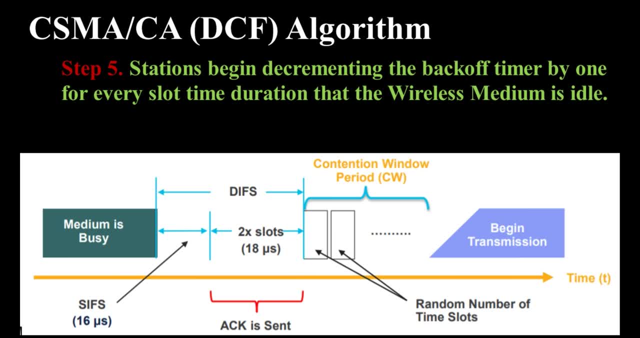 If station is wants only one of the four station values on the AC, they are guessing that the wireless medium is idle in decrementing the backoff timer by 1 for every slot-time duration and that the wireless medium is idle- Step 6.. After decrementing the backoff value to zero with an idle medium, a station may: 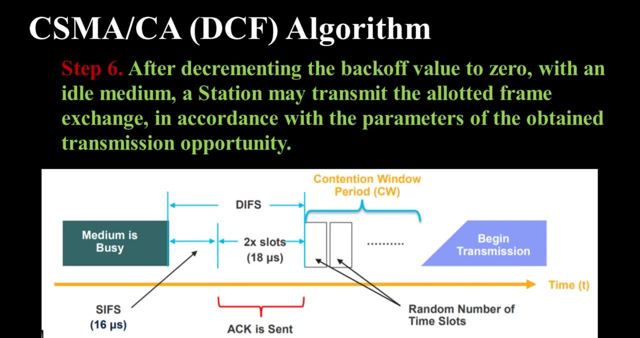 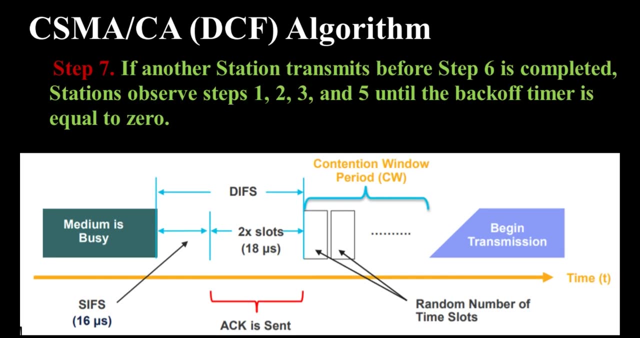 transmit the allotted frame exchange in accordance with the parameters of the obtained transmission opportunity- Step 7. If another station transmits before Step 6 is completed, stations observe Steps 1,, 2,, 3 and 5 until the backoff time timer are both wasте dialog. 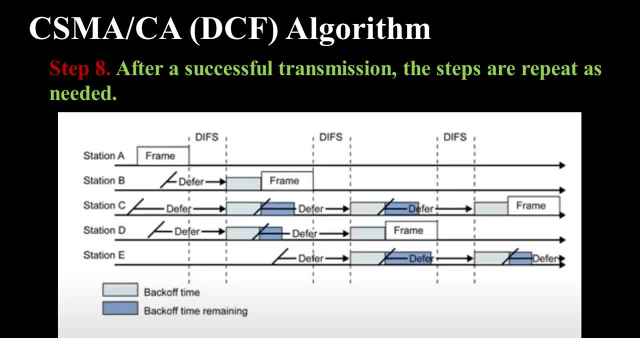 Step 6. After decrementing the backoff value to zero, a station may transmit the allotted frame exchange in accordance with the parameters of the obtained transmission opportunity. off timer is equal to zero. Step 8. After a successful transmission, the steps are repeated. as needed. 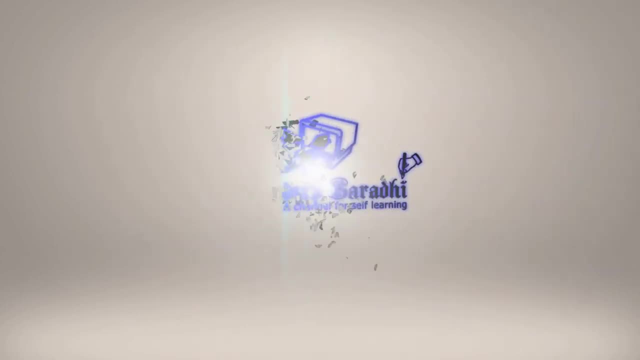 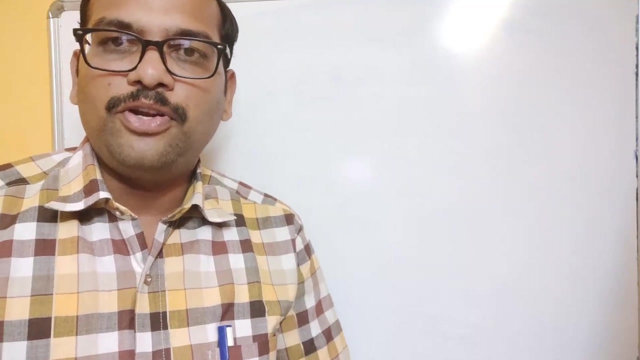 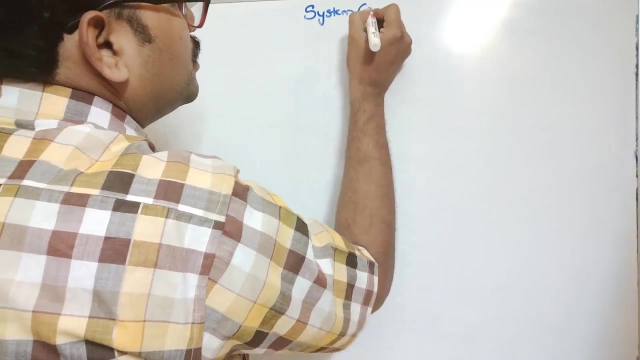 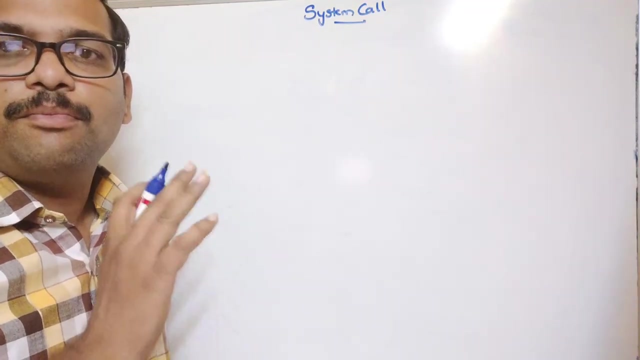 Hello friends, welcome back to our channel. So in today's session we'll discuss about one more concept in operating system, that is, a system call. So we'll see what is a system call and what are the need of this system call and how this system call works in operating system.